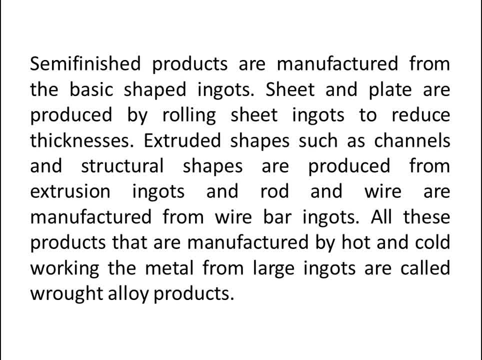 Semi-finished products are manufactured from the basic shaped ignots. Sheet and plate are produced by rolling sheet ignots to reduce thicknesses. Extruded shapes, such as channels and structural shapes are produced from extrusion ingots, and rod and wire are manufactured from wire bar ingots. All these 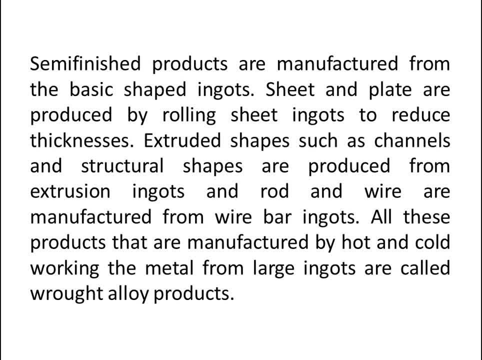 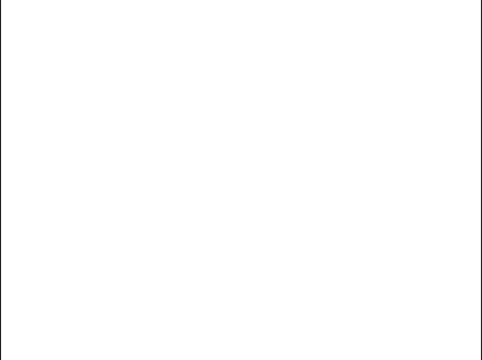 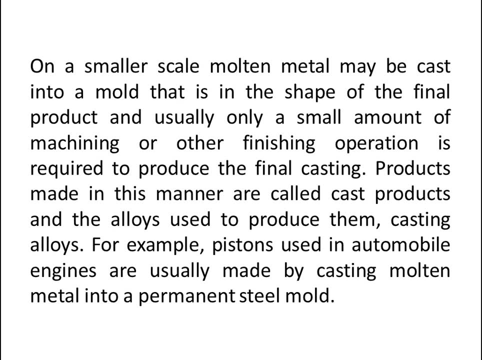 products that are manufactured from. these products are manufactured from the basic shaped ignots. They are manufactured by hot and cold working. the metal from large ingots are called RØT alloy products On a smaller scale, molten metal, may be cast into a mold that is in the shape of the final product. 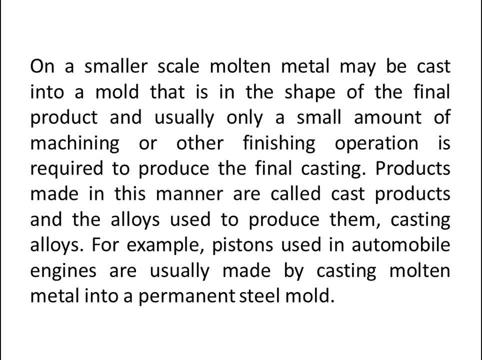 and usually with a small amount of machining or other machining operations, is required to produce the final casting. The mold that can be used will produce tortured products which will be used as molding material for the final casting of the molten metal. The molding material produced will be the molding material, The molding material that can be used in the production of that. 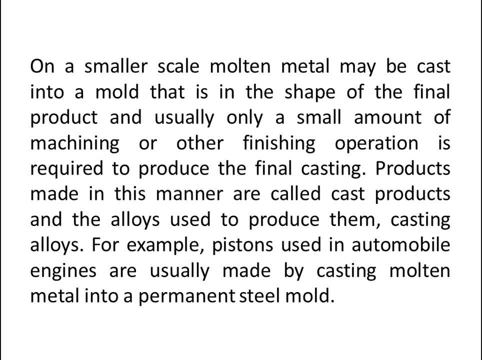 would be used for the final casting of the molten metal. The parts that are made in cold working- the metal from large ingots in this manner- are called cast products, and the alloys used to produce them casting alloys. For example, pistons used in automobile engines are usually made by casting molten metal into a 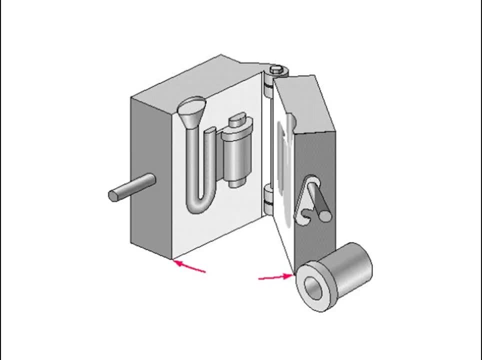 permanent steel mold and there is a mold and in the mold there is a cavity for producing any product and this is a cup and it is the way to run the material. So liquid is poured here and liquid come here and fill this gap and finally we get this product. and let's talk about hot and cold. 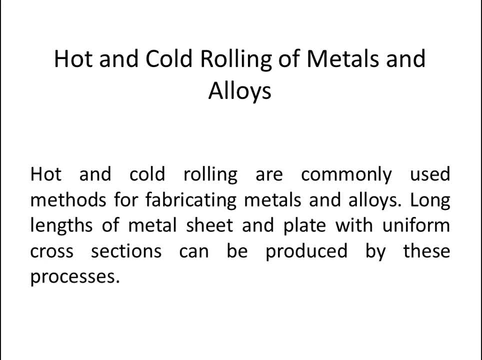 rolling of metals and alloys. Hot and cold rolling are commonly used methods for fabricating metals and alloys. Long lengths of rolling are commonly used methods for fabricating metals and alloys. Long lengths of rolling are commonly used methods for fabricating metals and alloys. and we call the most capacity of protectors from plastic devices for long length of시간 ofمن eso nos. Because the manufacture of polymers, in case of plastic currently used as sold haloys, are produced in these Egg of harmonic, the mankind or plastic raw materials, which are often artil. plastic materials also offer the 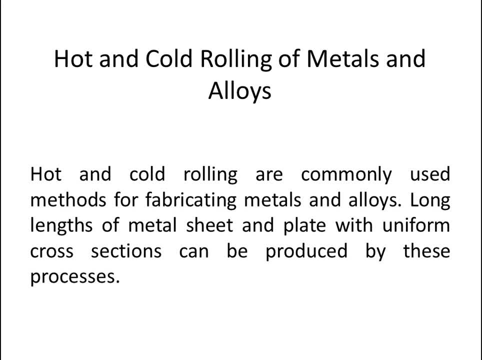 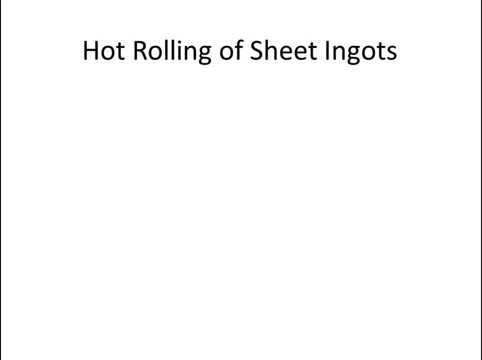 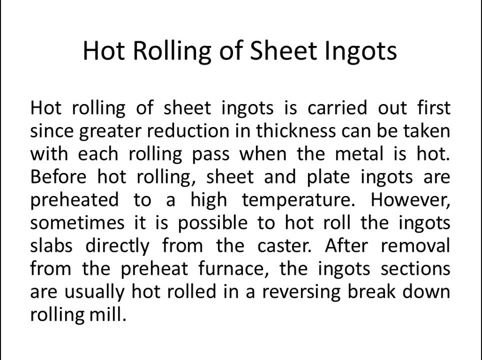 of metal, sheet and plate with uniform cross sections can be produced by these processes. Let's talk about hot rolling of sheet ingots. Hot rolling of sheet ingots is carried out fast, since greater reduction in thickness can be taken with each rolling pass when the metal is hot. 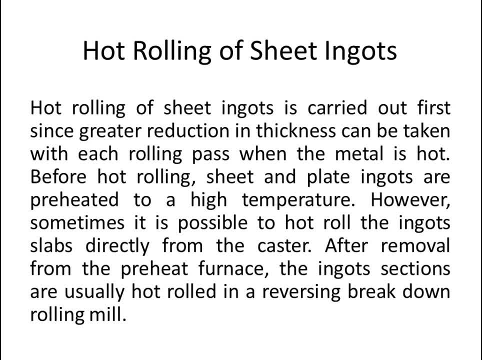 Before hot rolling. sheet and plate ingots are preheated to a high temperature. However, sometimes it is possible to hot roll the ingots slabs directly from the caster. After removal from the preheat furnace, the ingot sections are usually hot rolled. 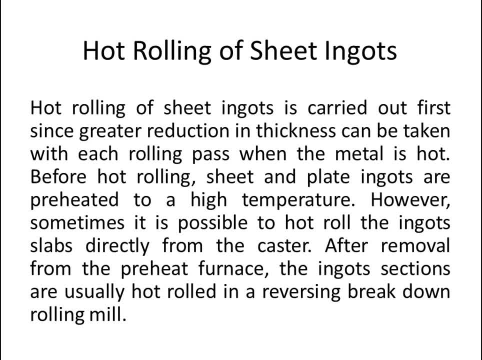 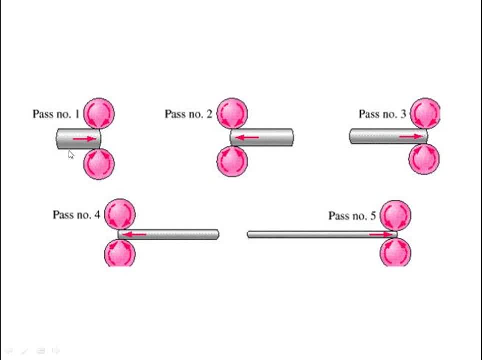 in a reversing breakdown rolling mill And there is a rolling, hot rolling, and this is a step one, so it is rolled here. so in step two we can see that it has been longer and thickness has reduced, and after step two that is step three or past. 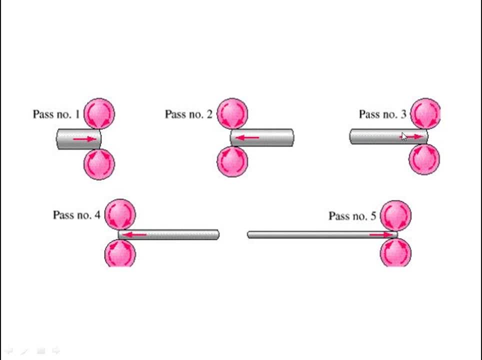 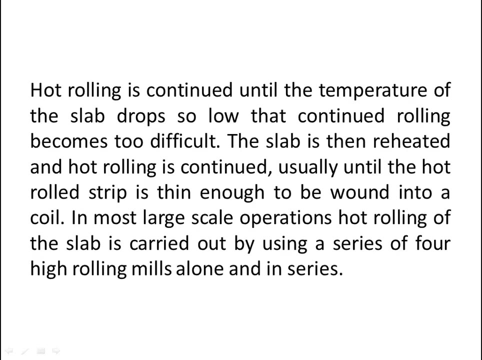 long three. so here also the length increased and thickness decreased. and after this one in fourth step the thickness also reduced and length increase. and in the fifth step we can see that the length has also increased and thickness has also reduced. Hot rolling is continued until the temperature of slab. 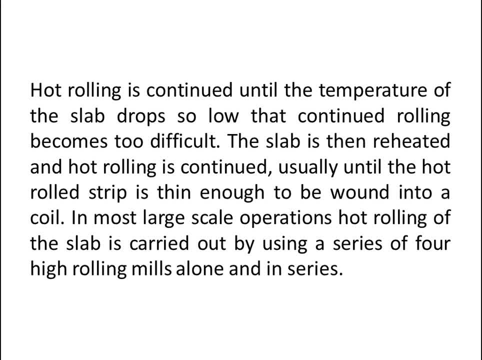 drops so low that continued rolling becomes too difficult. The slab is then reheated and hot rolling is continued, Usually until the hot roll strip is thin enough To be wound into a coil. in most large scale operations, hot rolling of the slap is carried out. 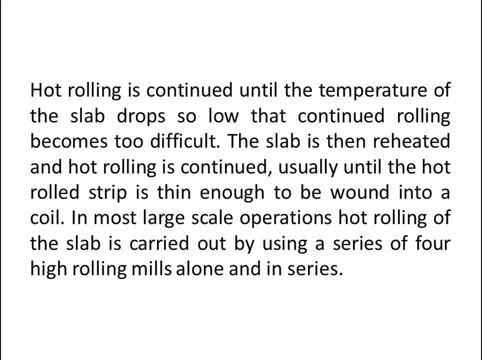 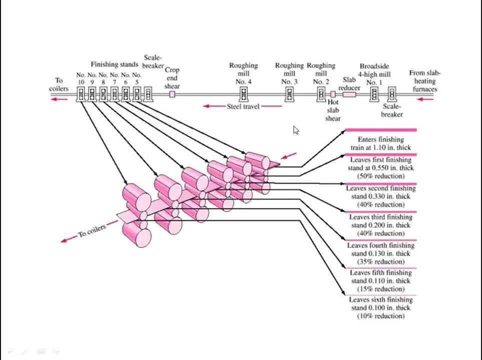 by using a series of four high rolling wheels, alone and in series, and we can see that there is a series of rolling and this is the first entering the sheet. so when this sheet comes here, the thickness is 1.1 inch and after passing this one, the thickness become 0.55 inch and the thickness reduced by. 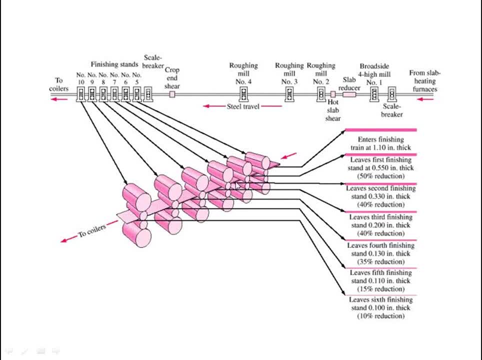 50%. and when the sheet leaves the second one, this is the second one and the thickness becomes 0.33 inch and forty percent reduction occurs in thickness. and when the sheet comes here that the third rule is passed, then the thickness becomes 0.2 inch. that means the 40 percent reduction occurs in thickness and the 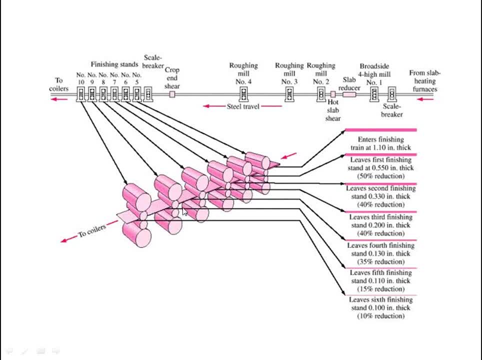 hand up. metals come here, then the thickness becomes 0.13 inch. that means that thickness is reduced by 35 percent. and when metal comes here, it comes here. then the thickness becomes 0.01 or 0.01 inch. that means the thickness reduced by. 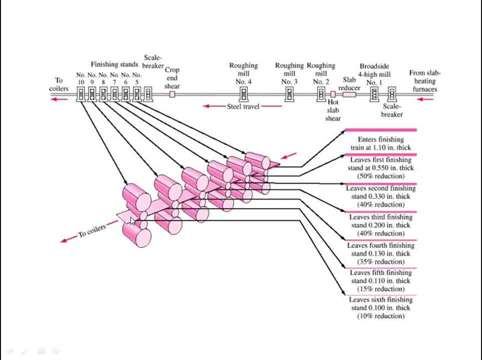 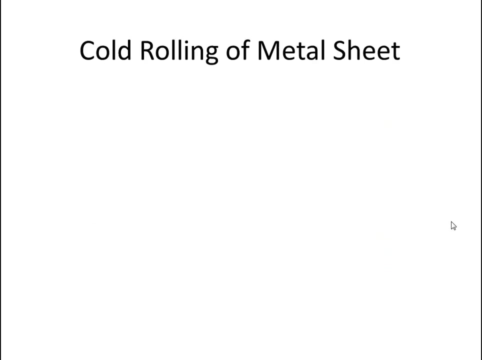 15 percent and when the coil come here, then the thickness becomes 0.1 inch and that means the thickness reduced by 10 percent. so we can see that the after rolling, after rolling the sheet metal, the sheet metal thickness becomes 0.1 inch to 1.1 inch. let's talk about cold rolling of sheet of metal sheet. 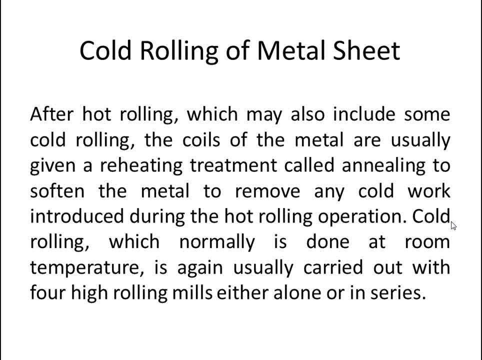 so after hot rolling, which may also include some cold rolling, the coils of the metal are usually given a reheating treatment, called annealing, to soften the metal, to remove any cold work introduced during the hot rolling operation. cold rolling, which normally is done at room temperature, is again usually carried out. 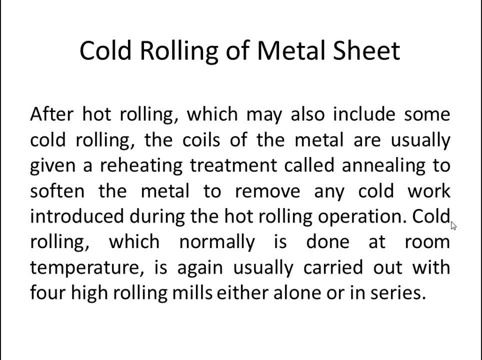 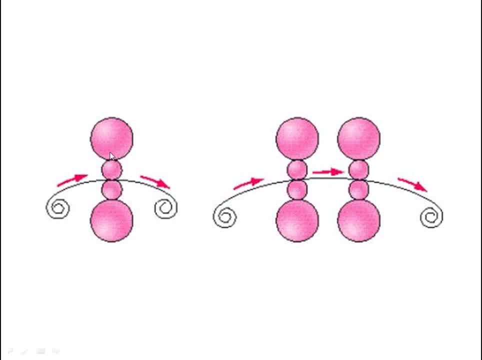 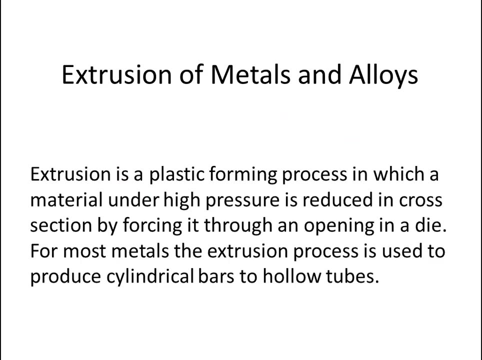 with four high rolling wheels, either alone or in series, and we take that, check, that see that there are four rollers and the thickness reduce here and also you can see that in series, so the thickness also reduced here. let's talk about extrusion of metals and alloys. extrusion is a plastic forming process in which a material under high pressure 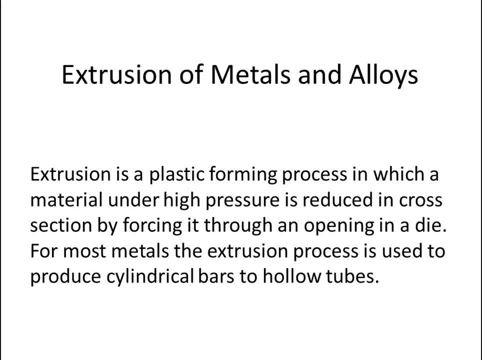 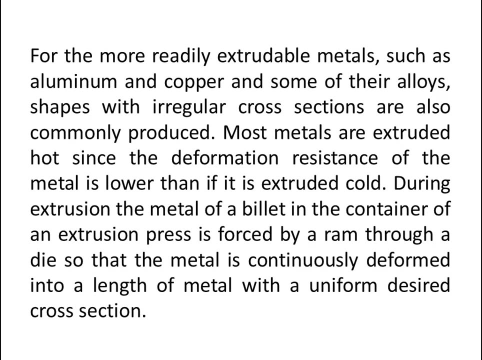 is reduced in cross section by: for by forcing it through an opening in a die. for most metals, the extrusion process is used to produce cylindrical bars to hollow tubes for the more readily extrude all metals such as aluminium and copper and some some of their alloys shapes. 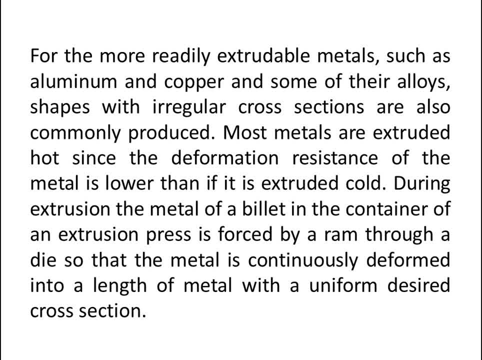 with irregular cross sections are also commonly produced. most metals are extruded hot, since the deformation resistance of the metal is lower than if it is extruded cold. during extrusion, the metal of a village in the container of an extrusion press is forced by a ram through a die so that the metal is continuously deformed into a length of metal with 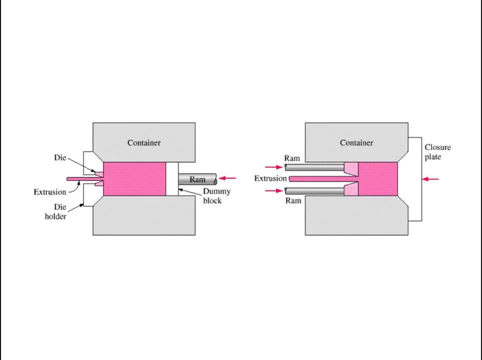 a uniform desired cross section and we can see here that this is the container and this is actually the material and this one is a die and this one is a die holder. destroy the die holder and the force is applied from here and these metals, from this metal. so you get this. 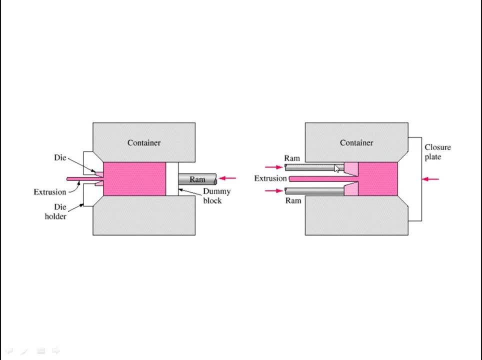 extrusion, thin parts, and also check this one. this is another type. so this one is the closure plate. it is closed, and this one is a metal and this one is the die, and here two ramps are here, so by this ram's force is applied and from this material finally we get this extrusion, this part. 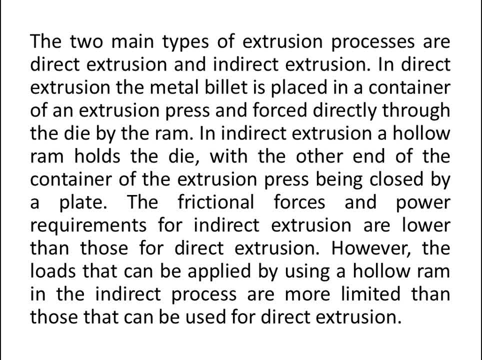 the two main types of extrusion processes are direct extrusion and indirect extrusion. in direct extrusion, the metal billet is placed in a container of an extrusion press and forced directly through the die by the ram. in indirect extrusion, a hollow ram holds the die. 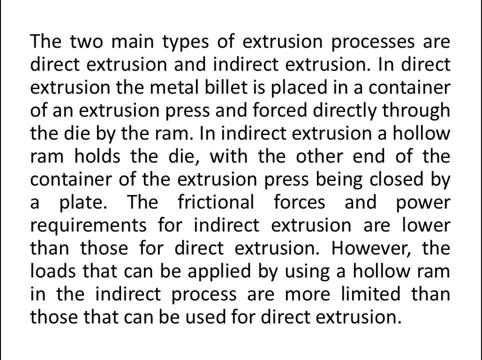 with the other end of the container of the extrusion place being closed by a plate, the frictional forces and the power requirements for indirect extrusion are lower than those for direct extrusion. however, the loads that can be applied by using a hollow ram in the extrusion plates will be. 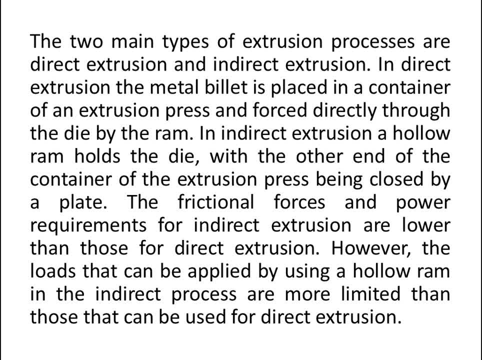 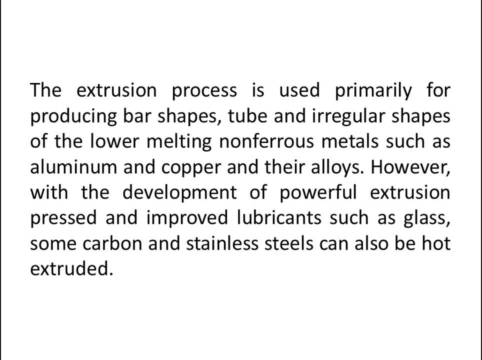 indirect process are more limited than those that can be used for direct extrusion. the extrusion process is used primarily for producing bar shapes, tube and irregular shapes of the lower melting non-ferrous metals such as aluminium and copper and their alloys. however, with the development of powerful extrusion paste and improved lubricants such as glass, 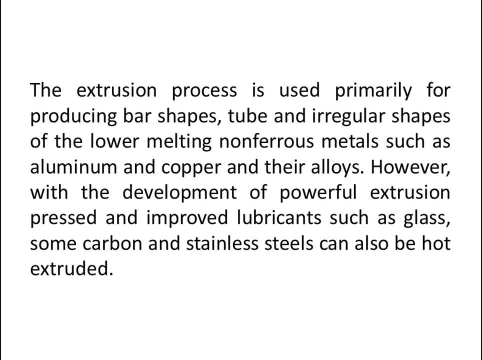 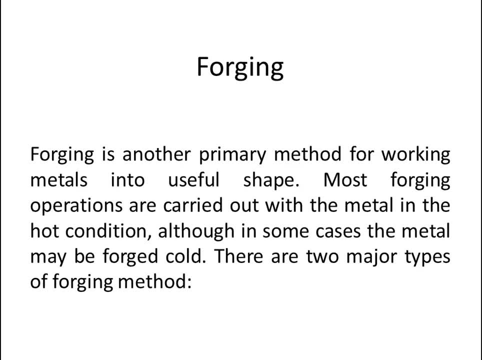 some carbon and stainless steels can also be hot extruded. let's talk about for forging operation. forging is another primary method for working metals into useful shape. most forging operations are carried out with the metal in the hot condition, although in some cases the metal may be forked cold. there are two major types of forging method. 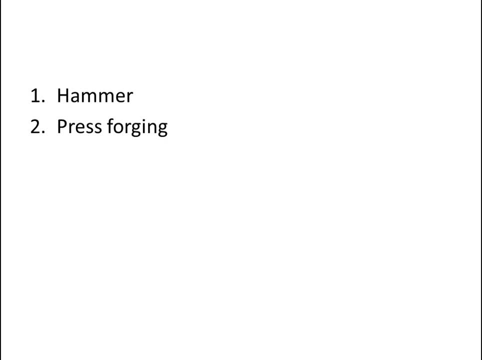 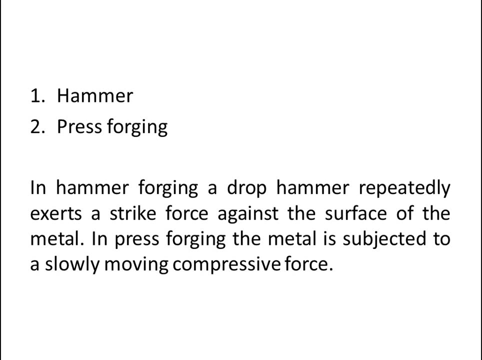 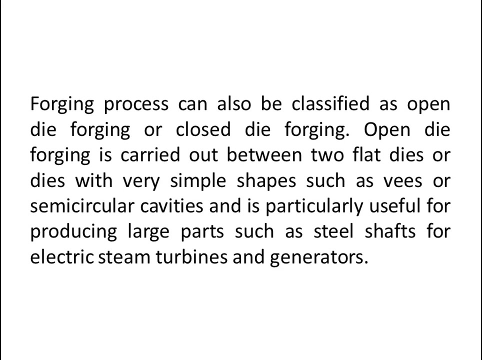 first one is hammer and second one is press forging. in hammer forging, a drop hammer repeatedly exerts a strike force against the surface of the metal. in press forging, the metal is subjected to a slowly moving compressive force. forging process can also be classified as open die forging or closed die forging. open die forging is: 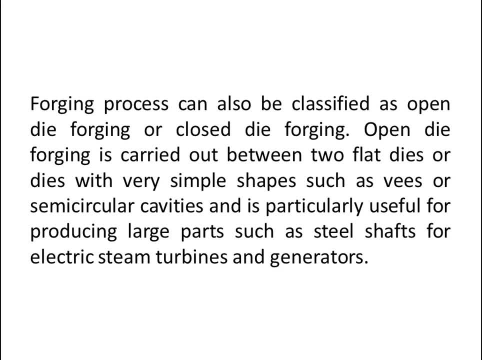 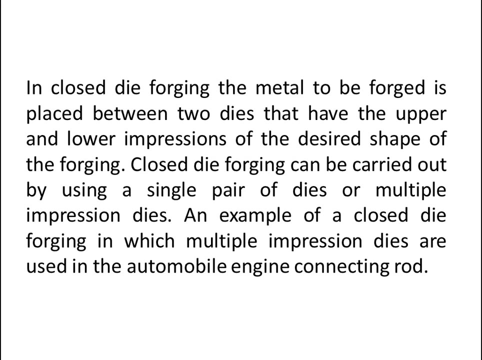 carried out between two flat dies or dies with very simple shapes such as v's or semi-circular cavities, and is particularly useful for producing large parts such as steel shafts for electric steam turbines and generators in closed die forging. the metal to be forked is placed between two dies. 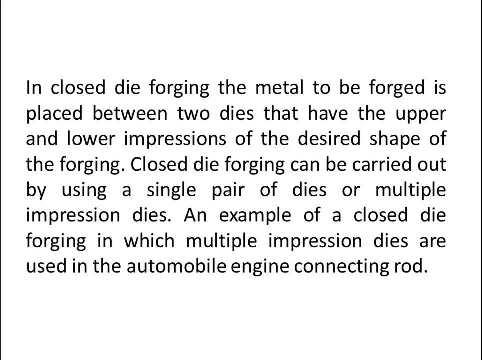 that have the upper and lower impressions of the desired shape of the forging. closed die forging can be carried out by using a single pair of dies or multiple impression dies. an example of a closed die forging in which multiple impression dies are used in the automobile engine connecting rod. 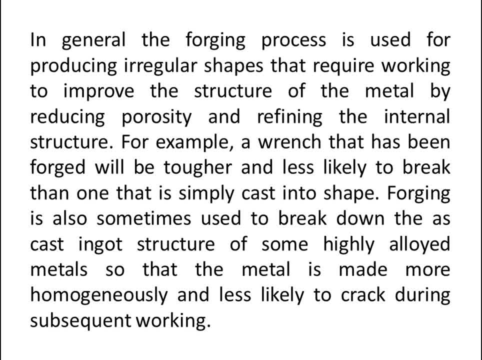 In general, the forging process is used for producing irregular shapes that require working to improve the structure of the metal by reducing porosity and refining the internal structure. For example, a range that has been forked will be tougher and less likely to break than one that is simply cast into shape. Forging is also sometimes used to break. 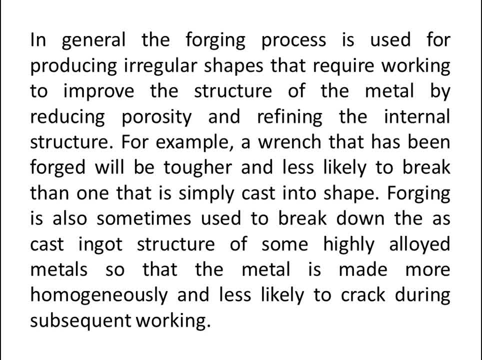 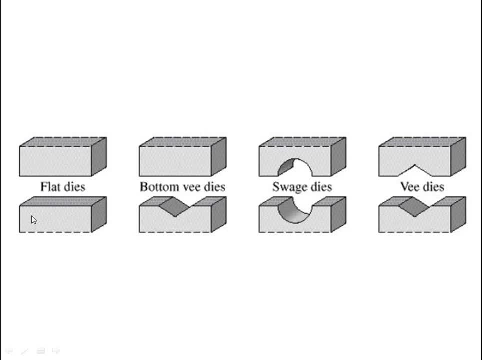 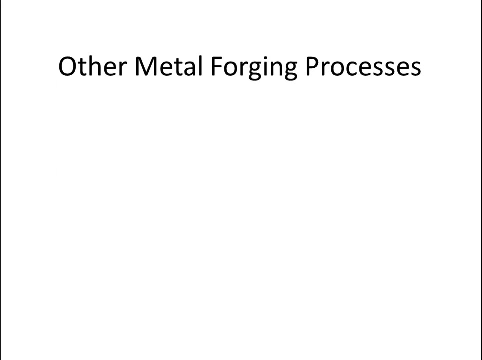 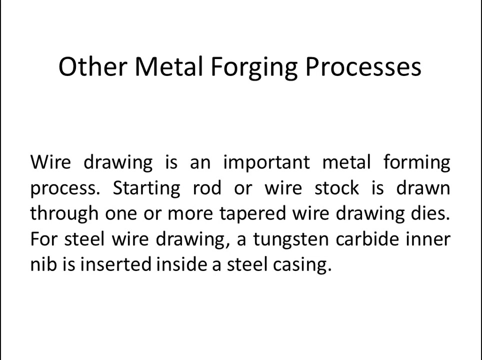 down as the cast ingot structure of some highly alloyed metals, so that the metal is made more homogeneously and less likely to crack during subsequent working. Let's talk about other metal forging processes. Wire drawing is an important metal forging process. Starting rod or wire stock is drawn through one or more tapered wire drawing. 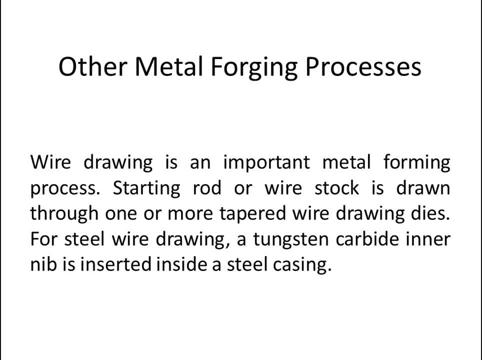 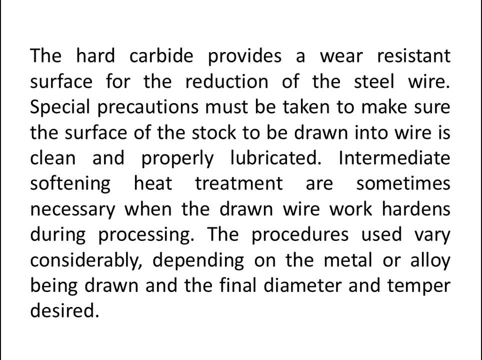 dies For steel wire drawing. a tungsten carbide inner nib is inserted inside a steel casing. The hard carbide provides a wire-resistant surface for the reduction of the steel wire. Special precautions must be taken to make sure the surface of the stock to be drawn into a wire is clean. 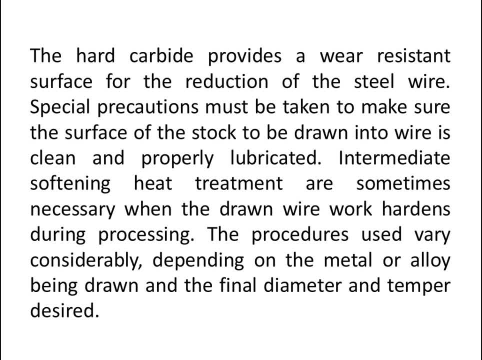 and properly lubricated. For steel wire drawing, a tungsten carbide inner nib is inserted into a steel casing. Intermediate softening heat treatment are sometimes necessary when the drawn wire work hardens during processing. The procedures used vary considerably depending on the metal. 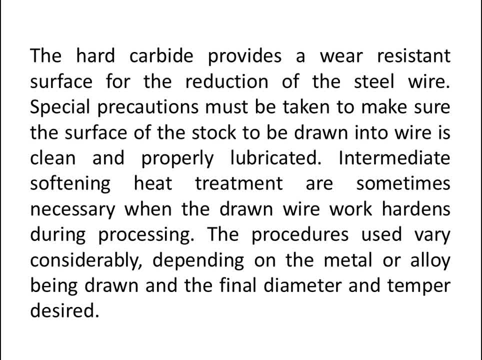 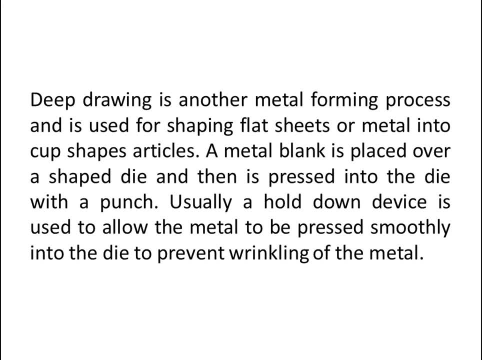 or alloy being drawn and the final diameter and tamper desired. Deep drawing is another metal forming process and used for shaping flat sheets or metal into cup shapes articles. a metal blank is placed over a shaped die and then is pressed into the die with a punch, usually a hold down device.